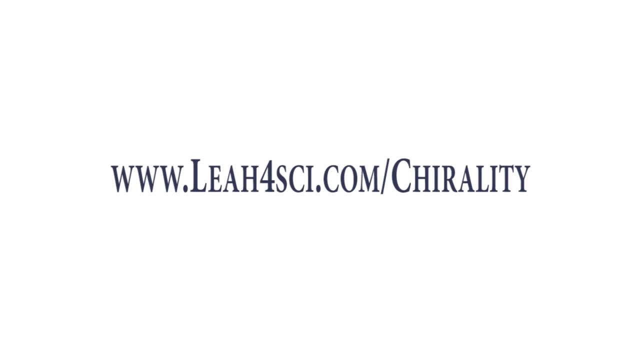 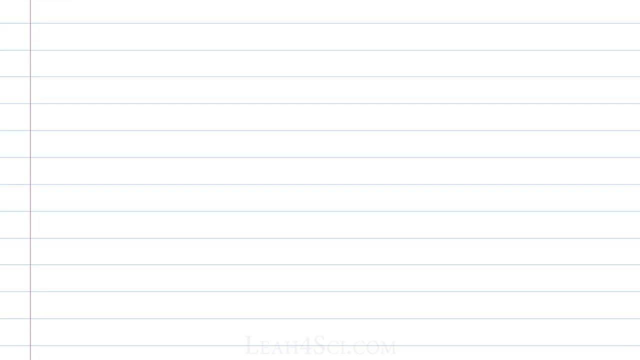 video series, practice quiz and cheat sheet by visiting leah4scicom. slash chirality Before we look at the math, what is enantiomeric excess or optical purity? We've already discussed that if you have a pure R or pure S sample, these are going to be optically active by 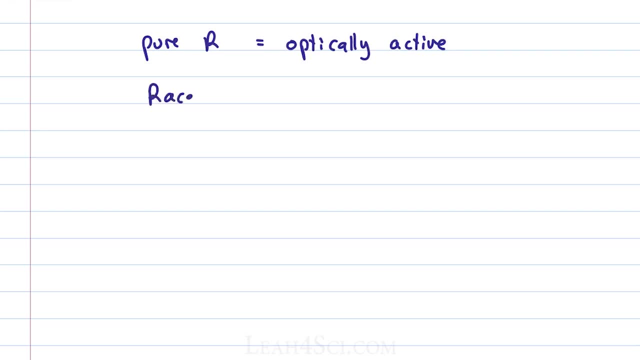 turning light in one direction or the other. And if you have a racemic mixture it'll be optically inactive because every molecule trying to turn light to the right will be cancelled out by another one turning it to the left. But these are extremes: 100% R or 100% S versus 50% R, 50% S. But what happens if you have a sample? that is not pure, but not quite 50-50?. You're still going to have some optical activity, but it won't be quite as strong as the pure sample. Let's say the pure sample of some molecule has a specific rotation that is equal to positive. 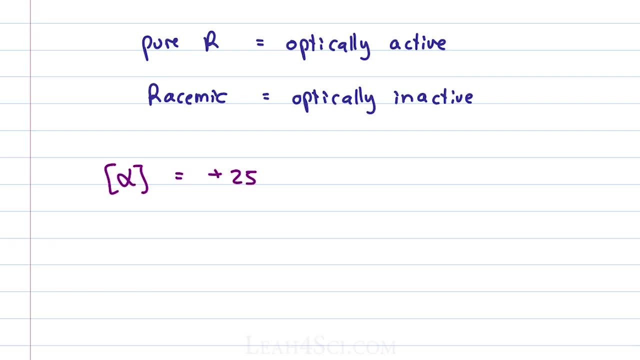 25. It turns light 25 degrees to the right, and that would be for the R enantiomer and that means the S enantiomer should be equal to negative 25. If we mix them together, so that would be 50-50 R and S. we get an alpha that is equal to zero degrees, because it doesn't. 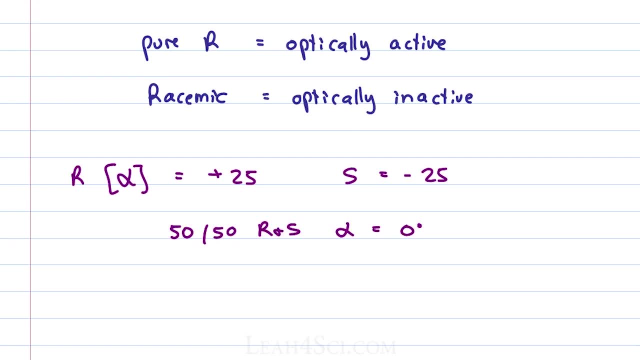 turn in either direction. R and S cancel out. But then what happens if I give you a sample that has some mix of R and S but the alpha comes out to be negative 12.5 degrees? That means it's turning to the left, but not quite as much as we would expect for a pure sample. 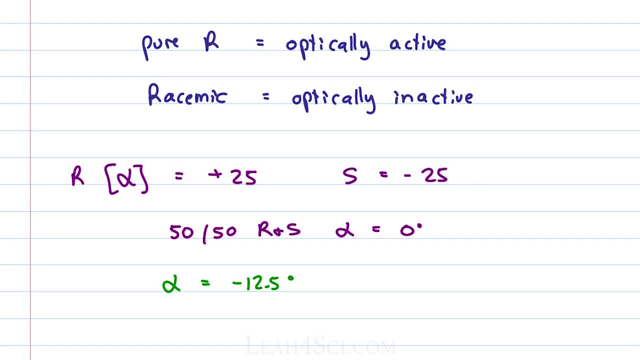 Let's approach this from a logic perspective first, and then we'll look at the calculation. Sometimes on your exam you're simply asked which one dominates R and S, and for that you want to draw a quick mental map and say, if I have the extremes, I'm going to have. 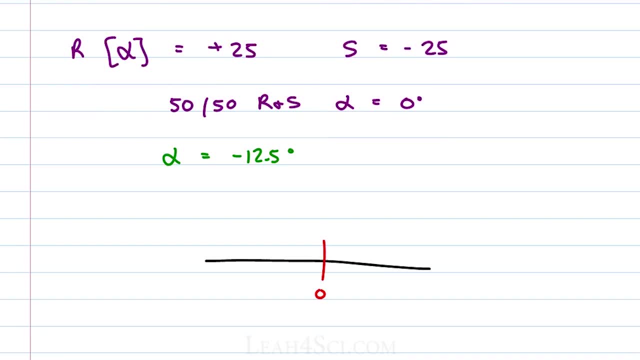 S and zero is in the middle. negative 25 would be pure S, positive 25 would be pure R. If the observed rotation is somewhere in this direction, at negative 12.5,, it's halfway between racemic, where they both cancel, and pure, where you have only S. 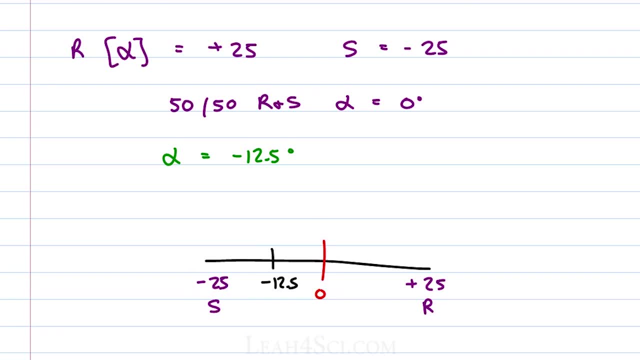 So if we had to guess, we'll say first of all, S definitely dominates, We have more S than R And we probably have about 75% S and 25% R. This is helpful if you have a multiple choice question and you just need a direction where it's extremes or somewhere in the middle and 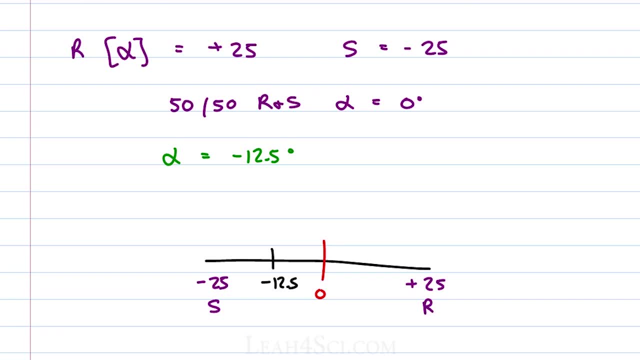 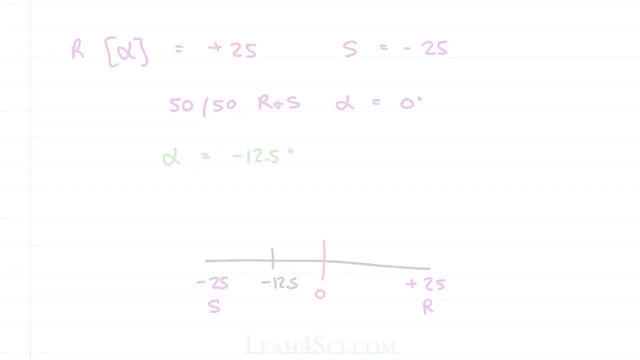 you quickly rule out the R as being the dominant. But what if we want to know exactly how much? Before we go into the mathematical answer, let's take a look at what is happening. Say we have a solution where R is blue and S is green. 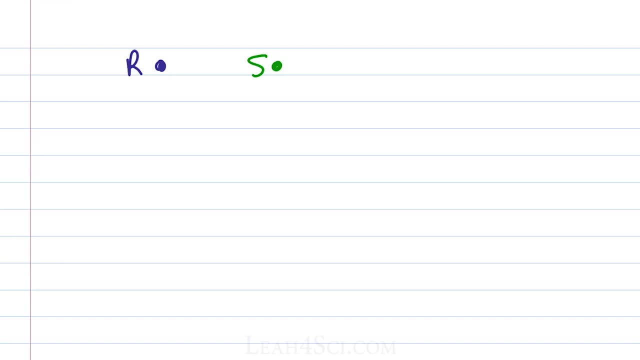 And I want to find out the optical purity or enantiomeric excess. And in this solution I have three blue and seven. green Purity means what is not cancelled out by the other one and excess means after everything is cancelled out, it's what is left over. So 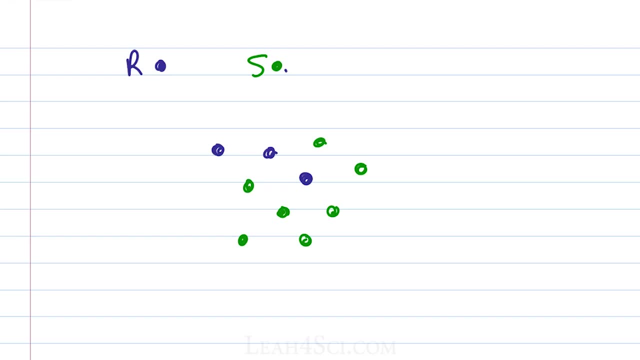 optical purity and enantiomeric excess is kind of the same thing. The way I would figure this out is say that for every blue R, one green S would be negative 25 and negative S cancels. So even though we have seven green and three blue, one green and one blue cancel. 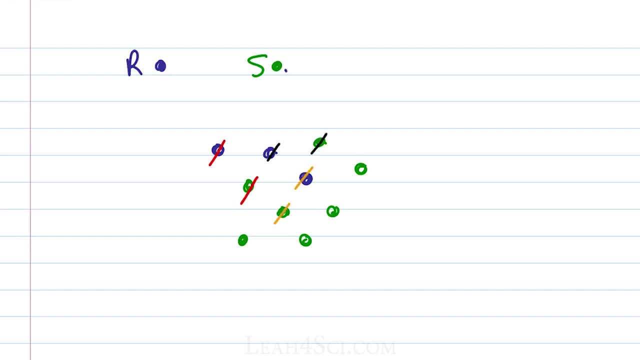 a second blue and green cancel and a third blue and green cancel. There is no more blue to cancel the green, so anything that could have cancelled was taken out of the way. That leaves us with one, two, three, four green left over with nothing to cancel. That means 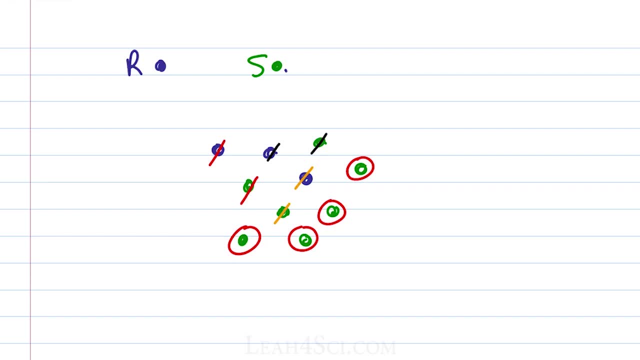 going back to the polarimeter, if light is coming through this system, every time this blue one tries to rotate light in one direction, the green one rotates it back in the other direction. Every time this blue one tries to turn light, the green one cancels it out. 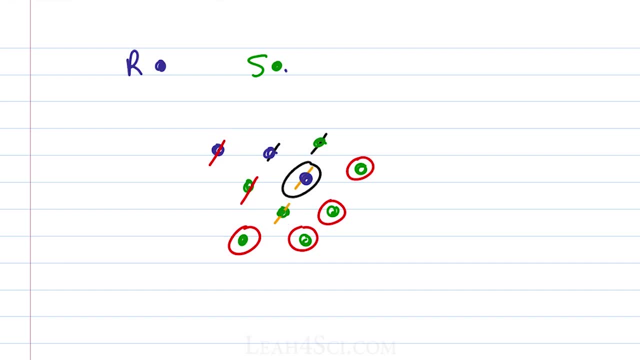 Every time the blue one tries to turn light, the green one cancels it out, and then the remaining green. when they try to turn light, we have no more R to cancel it out, because the R is completely outnumbered by eight. So the green will win and force light in the direction that they would typically go. but 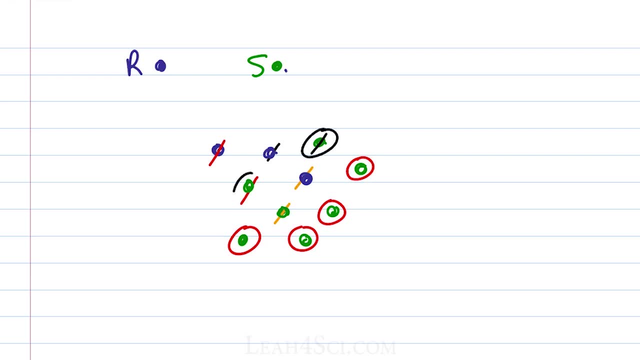 not quite as much, because half the green, or nearly half the green in this case we're not turning light to turn it, but simply to undo what the R is doing. So if we look at the excess in this case, we have a total of ten, and that means ten would equal to a hundred. 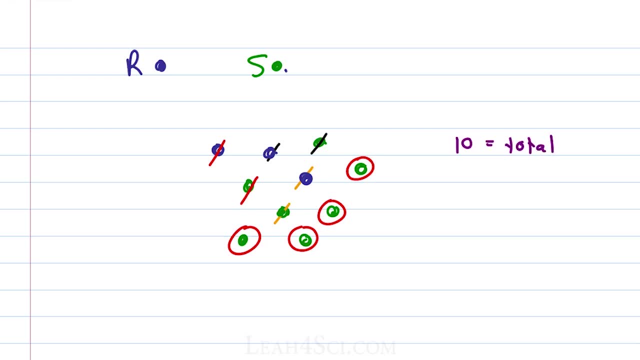 percent of the solution. but then, in this specific solution, three out of ten is R. that means we have thirty percent R, seven out of ten or seventy percent S, but for every R we need to cancel S. So what did we do For every R we took? 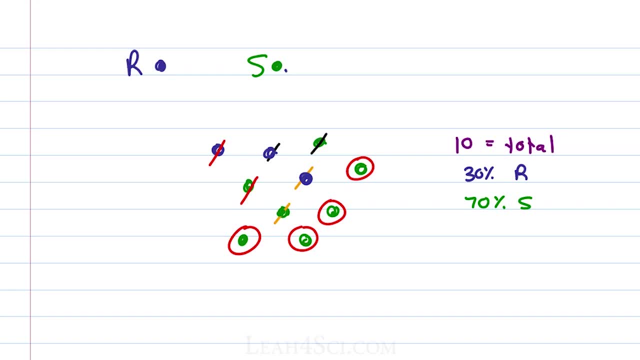 one S, we simply subtract and we say that if we have seven total S, but of the seven we have to take out three because we have three R and we need to cancel. that leaves me with a net of four. So we have four S capable of doing S rotation. 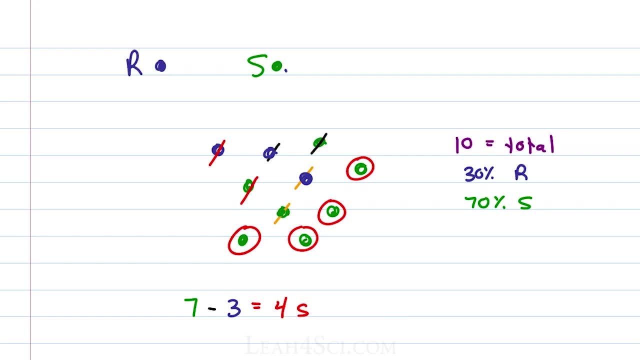 Your professors will show you different ways to calculate an anti-americ excess. I just like to go with high minus low, because I don't wanna deal with negatives if I don't have to. The higher percent, the greater concentration is S at seventy percent minus the lower concentration. 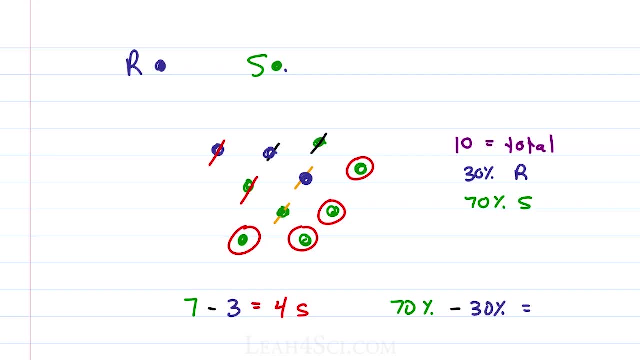 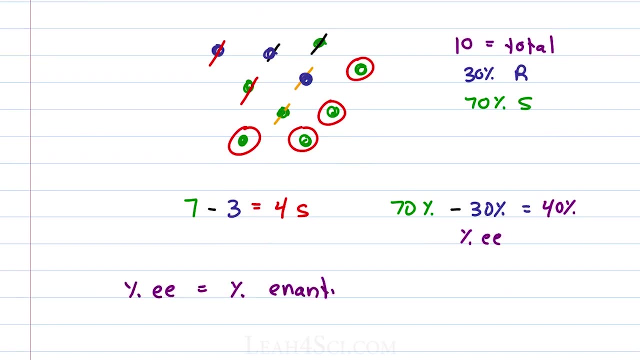 is thirty percent R, which leaves me with forty percent, an anti-americ excess, or percent EE, or an anti-americ excess. It's what remains of the an anti-amer that we had more of to begin with, In this case forty percent. Another way to look at this is of the seventy percent. 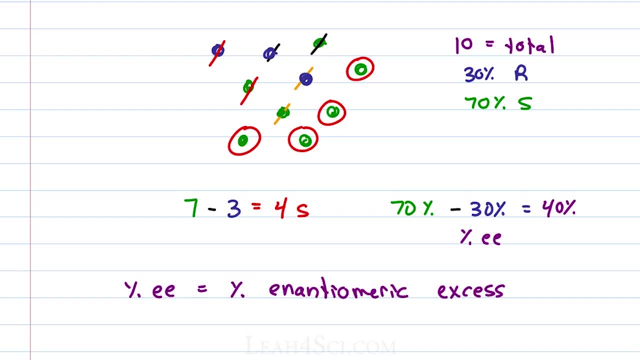 S. thirty percent is not pure because it's canceling out R, but what's left over is pure S, with nothing to battle, and that means we have an optical purity of forty percent, because that's what's left over and not rivaled by any left over. 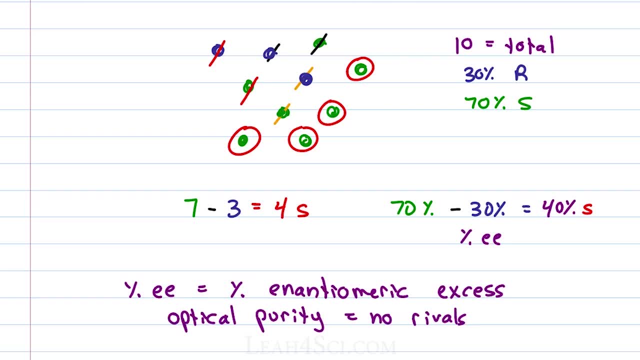 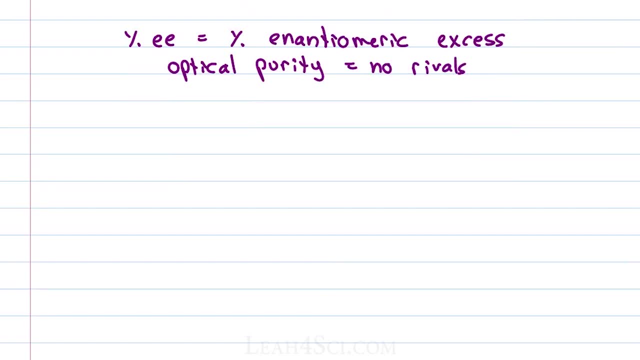 any leftover R. This was pretty simple, but what if you're asked this question in terms of observed rotation? Say, you're given the observed rotation and you're told it should normally have a different value, how do you calculate it? Which brings us to the second of a tiny number of equations you have to know in organic. 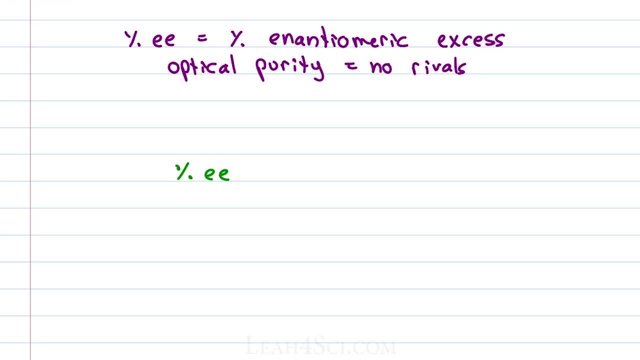 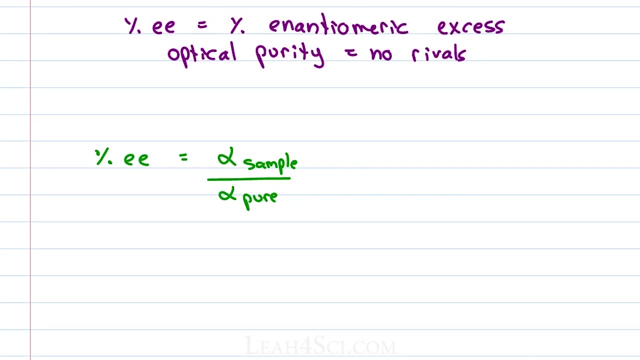 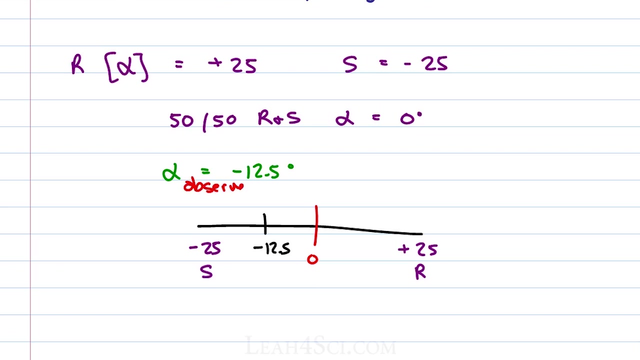 chemistry, and that's as follows: Percent enantiomeric excess or percent purity is equal to alpha of the sample or alpha observed- whatever you get out of your polarimeter- divided by alpha of the pure solution. Since we're looking for a percent value, we then multiply by 100%. In our first example, we are told that 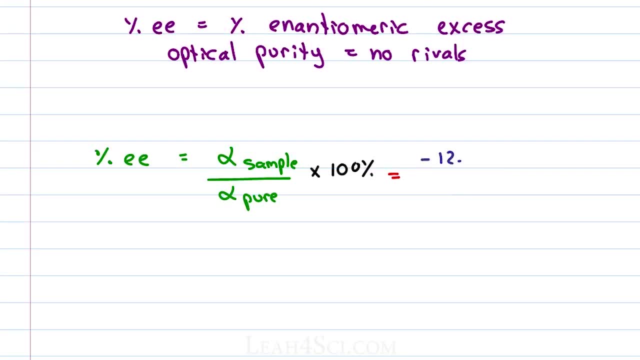 the alpha observed is equal to negative 12.5 degrees and the alpha pure was negative 25 degrees. If we punch this into the calculator, we have negative 12.5 divided by negative 25, notice that the negatives will cancel out and we get 0.5. But 0.5 is not a percent, so 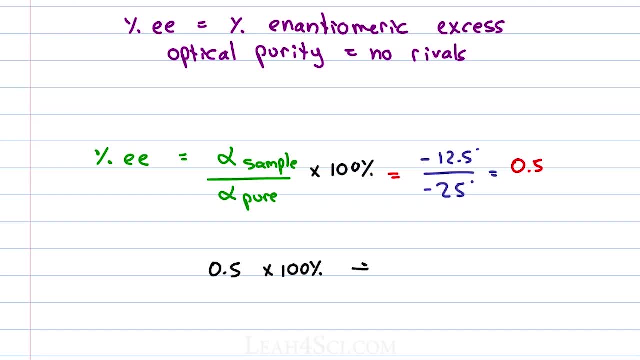 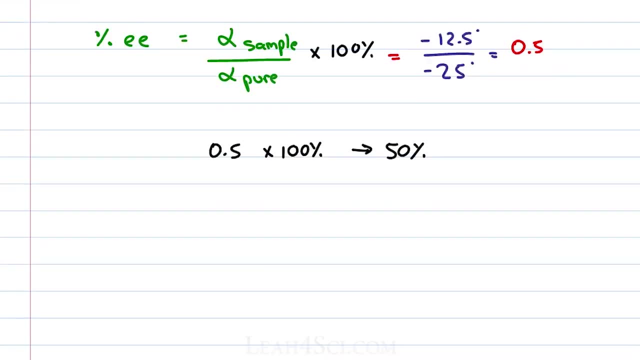 remember you have to multiply this by 100 and that gives me 50%. What is 50%? An enantiomeric excess. So don't think of this as 50% S. it's 50% S. It's 50% extra of your S. So if we take the entire sample and set that to a, 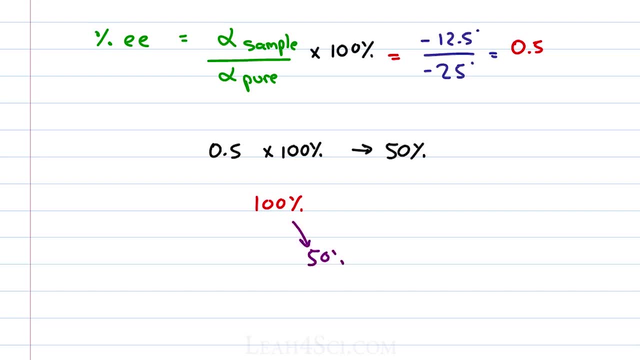 hundred percent. in that sample we have 50% pure S and then the other 50% is going to be racemic. For a racemic mixture you have half and half, so that would be 25% R and 25% S. From this we can then get the total and say we have: 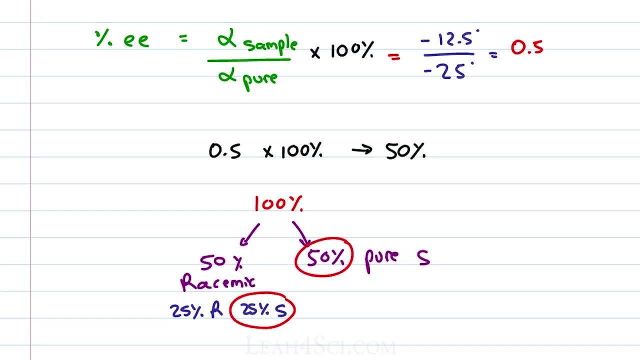 25% S, cancelling 50% S, that is pure for a total of 75% S in solution and, of course, 25% R in solution Again. what did we do here? We figured out the percent optical purity or the percent enantiomeric excess. what is left over After I compare the R and S that cancels? 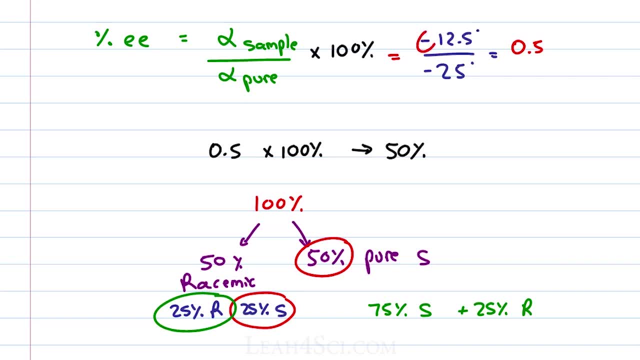 out what is left over. we know that it's S because it's the same sign as the pure S, So it has to be an excess of the S enantiomer and that's 50% of the solution. that is pure S, with nothing to cancel out. 50% is pure S. what is the? 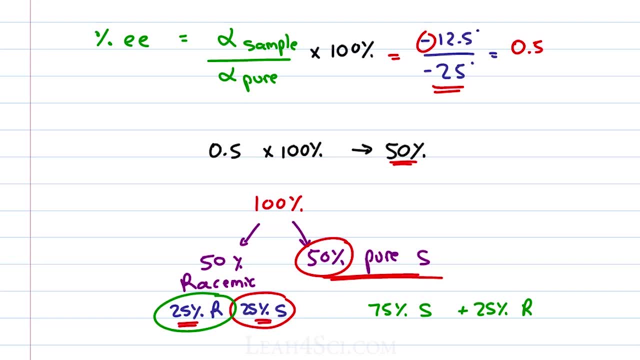 remainder of the solution- 25% R and 25% S, simply dividing it by two. But then we have to take everything back to consideration to get a hundred percent. We have 25% of the S cancelling R, 50% of the S, that is. 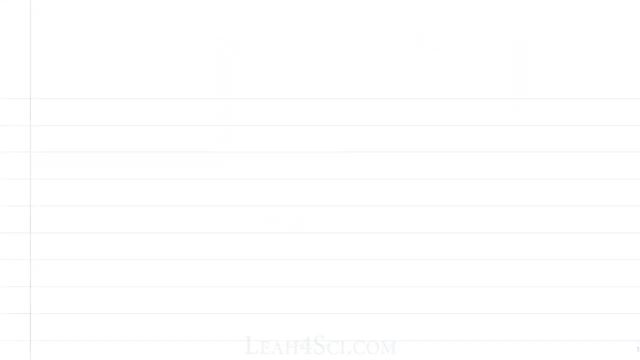 pure, and that gives us 75 and 25.. Let's do one more example because I know it's a little confusing. Say: we have another molecule where R is equal to negative 37.5 degrees and S is equal to positive 37.5 degrees. Recognize that the 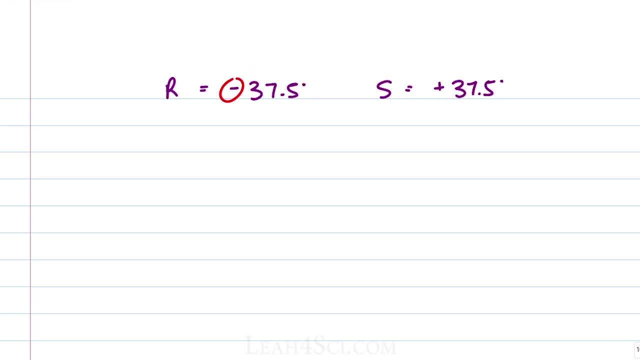 absolute value is exactly the same, but in this case R happens to be negative, S positive, because they can change depending on the molecule. But I tell you that in a certain sample, the observed rotation of the sample is equal to negative 13.7.. What is the enantiomeric excess? So let's set it up. 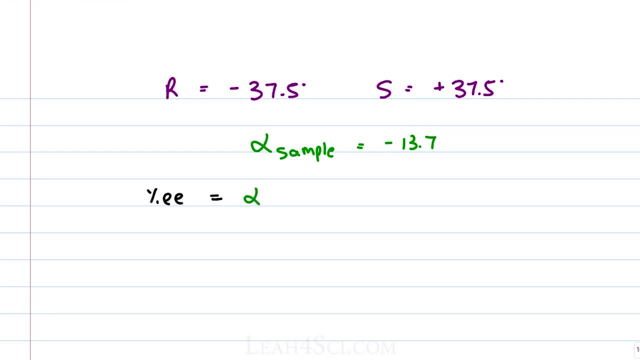 Percent enantiomeric excess is equal to alpha sample over alpha pure. In this case the sign is negative, so we know that it's going to be R. So it's percent enantiomeric excess of R And then alpha sample is equal to negative 13.7.. Alpha pure is equal to: 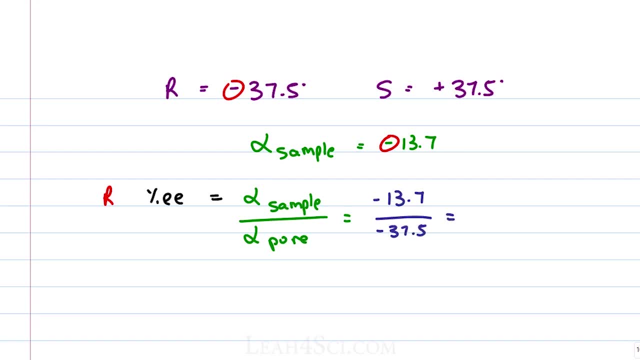 negative 37.5.. Punch that into the calculator. The negatives cancel out. We're just looking for a percent value. Punch this into the calculator and you get 0.365.. Don't forget to multiply this by a hundred percent, which gives us 36.5. 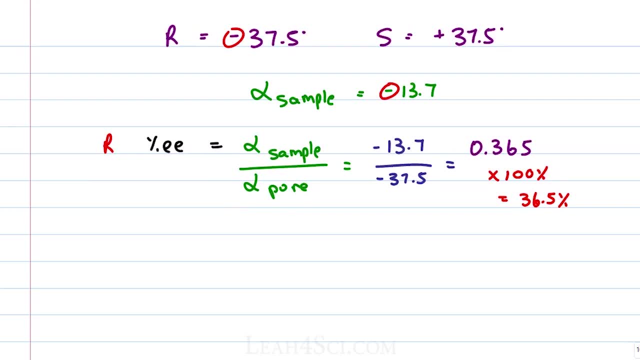 percent enantiomeric excess. What does this mean for the total R and the total S? If we have a hundred percent total, we know that we have 36.5 percent unopposed R and the remainder, which is a hundred minus 36.5, which is equal to 63.5 racemic. 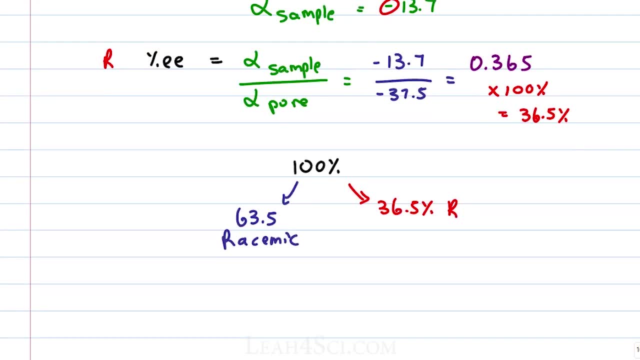 We have to split this in half, because it's half R and half S. So divide by two gives me 37.75, which will round up to 31.8, and that gives me 31.8 of R and 31.8 of S. 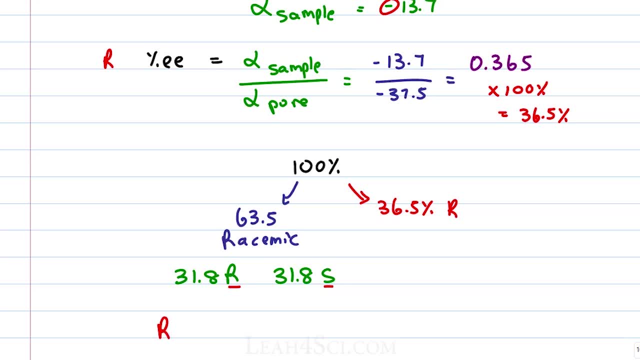 For a total solution of R, which is equal to the racemic portion and the enantiomeric excess portion. just add them up and that is equal to 68.3 percent, and, of course, 31.8 percent of S, For even more.